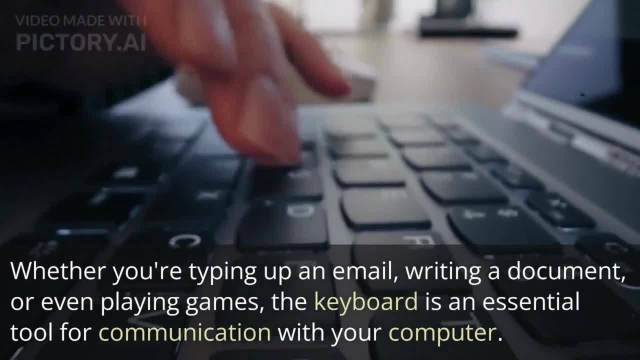 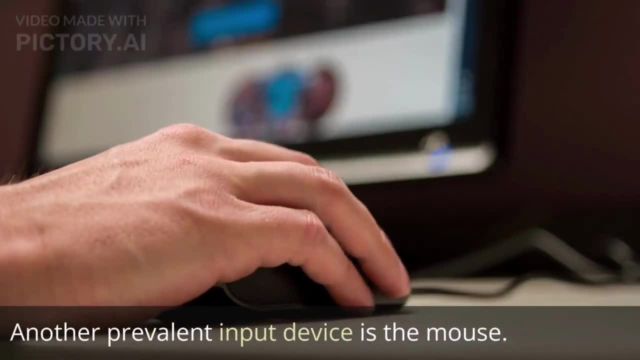 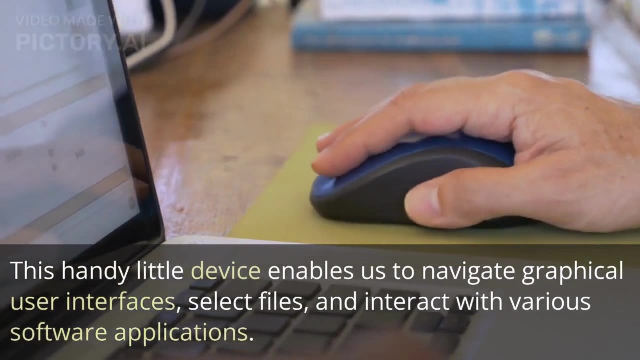 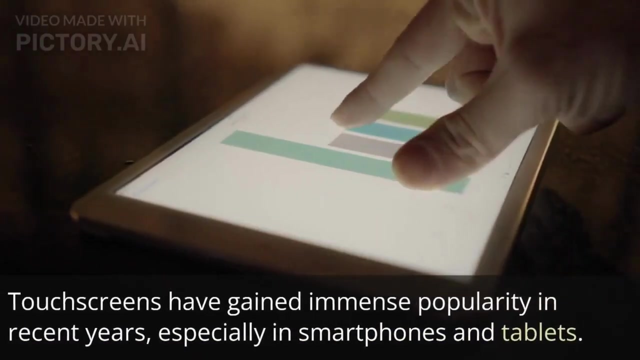 the keyboard is an essential tool for communication with your computer. Another prevalent input device is the mouse. This handy little device enables us to navigate graphical user interfaces, select files and interact with various software applications. Touch screens have gained immense popularity in recent years. 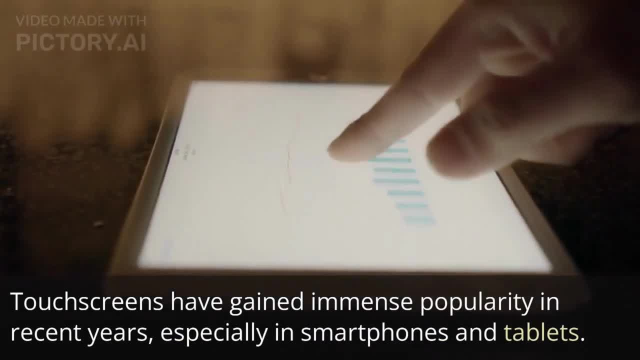 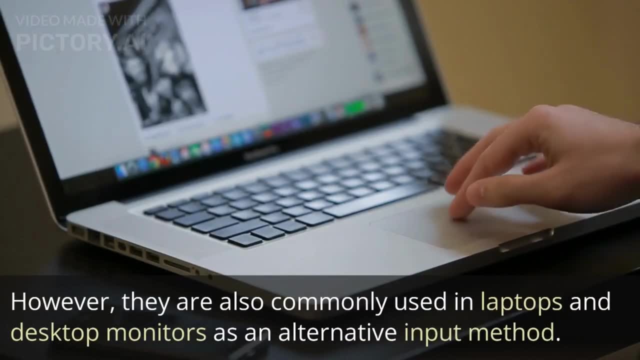 especially in smartphones and tablets. However, they are also commonly used in laptops and desktop monitors as an alternative. Do you want to start using an einfach mouse to use difficulty with the touch screen and select your favorite different keyboard? The mouse is so easy to use with any type of keyboard. 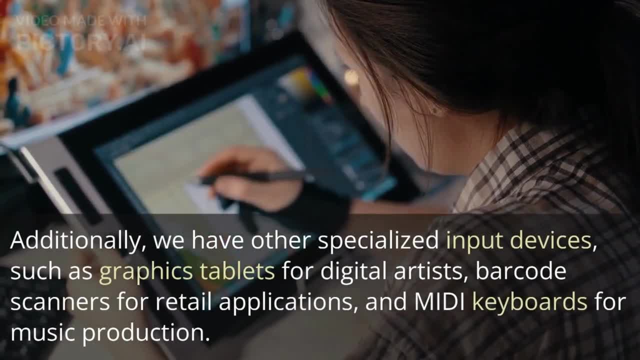 and this is why we use digital devices. the most popular are those that work with other digital devices. It's more likely that you'll use more than one. The most common type of devices are the screen cameras, the mouse and the mouse having two, etc. 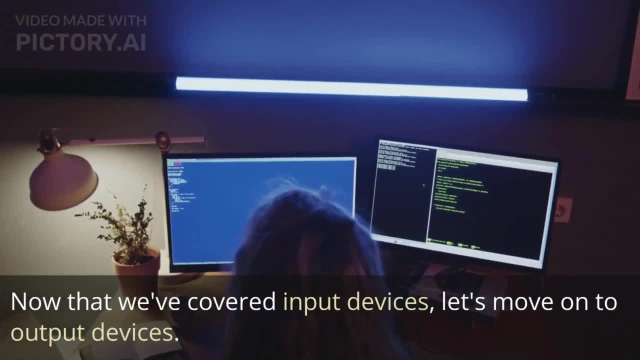 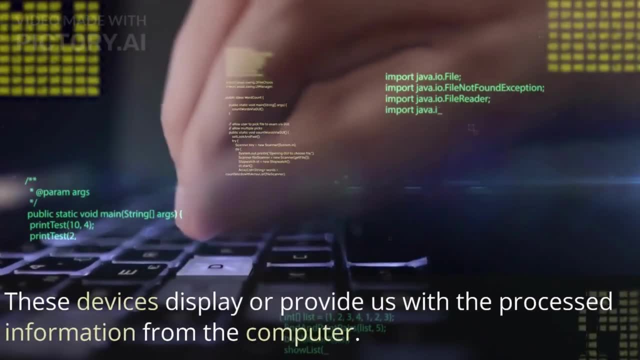 The smartwatch can be used as a standard keyboard. the mouse has a camera, which can be used for games. the mouse can be used as a monitor and the mouse can be used as a mouse with a main mouse. The婶tle features are similar in that they feature different keys. 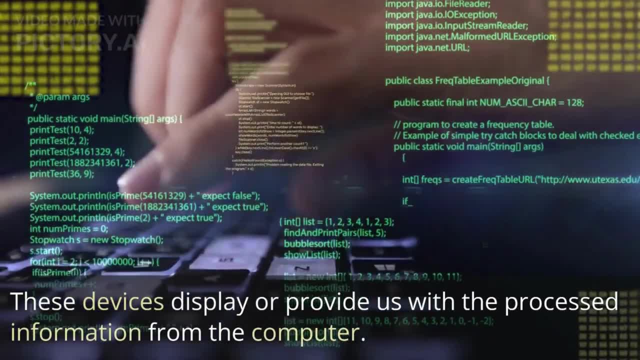 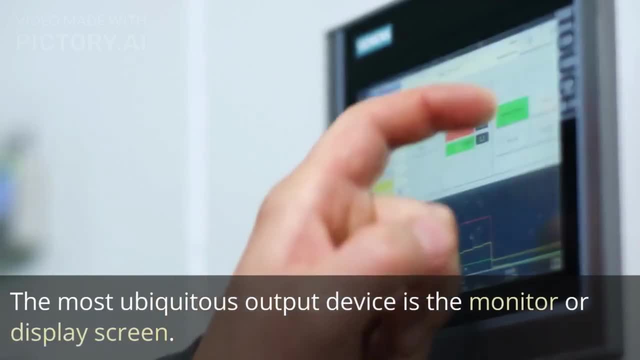 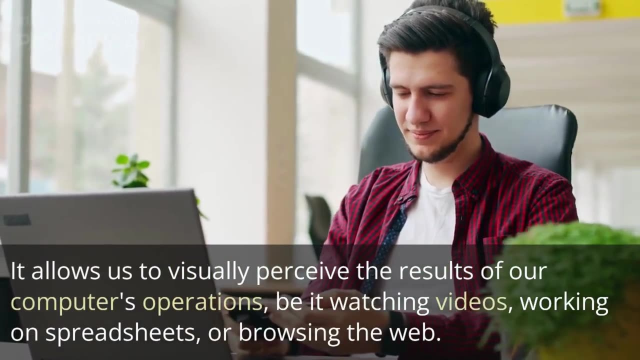 which can be used to unlock or unlock products information from the computer. The most ubiquitous output device is the monitor or display screen. It allows us to visually perceive the results of our computer's operations, be it watching videos, working on spreadsheets or browsing the web. 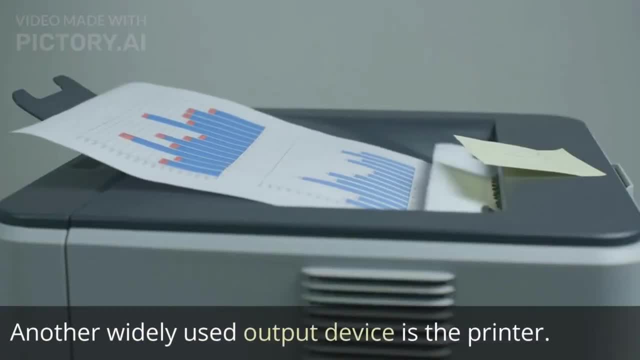 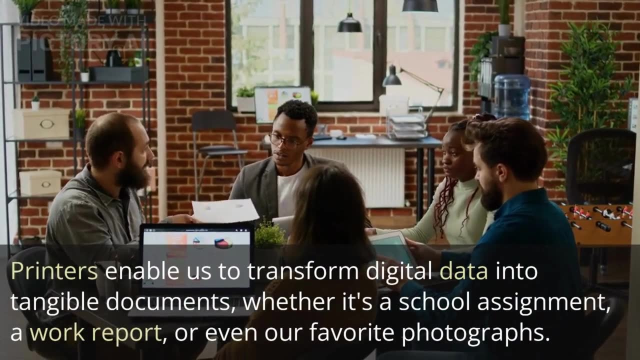 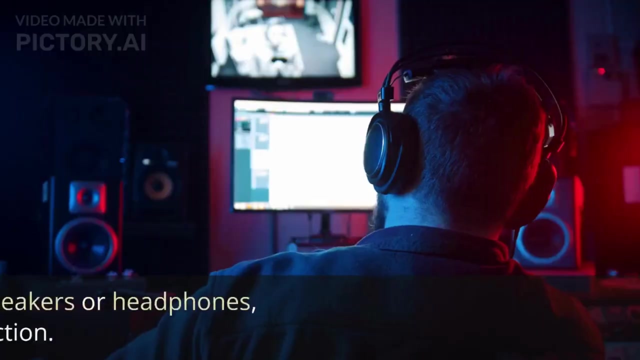 Another widely used output device is the printer. Printers enable us to transform digital data into tangible documents, whether it's a school assignment, a work report or even our favorite photographs. Audio output devices such as speakers or headphones are essential for sound reproduction. 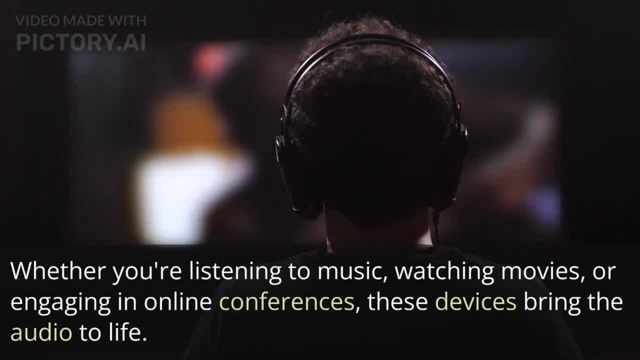 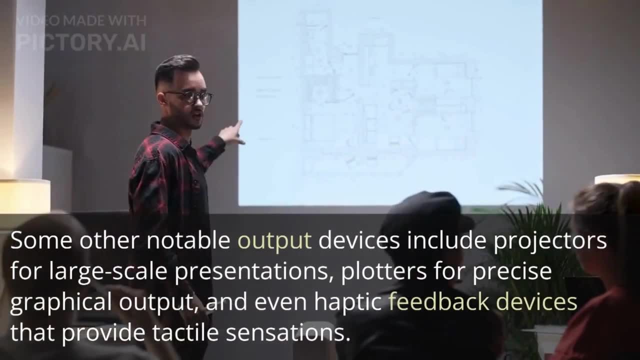 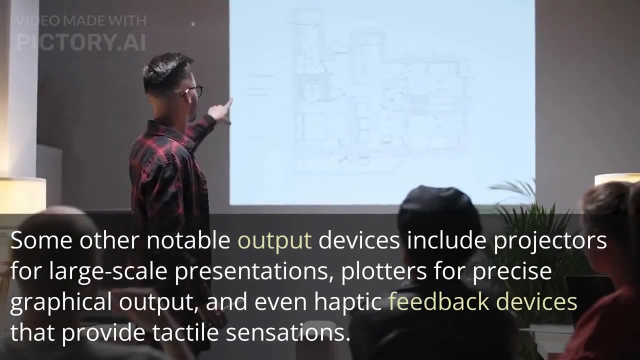 Whether you're listening to music, watching movies or engaging in online conferences, these devices bring the audio to life. Some other notable output devices include projectors for large-scale presentations, plotters for precise graphical output and even haptic feedback devices that provide tactile sensations. 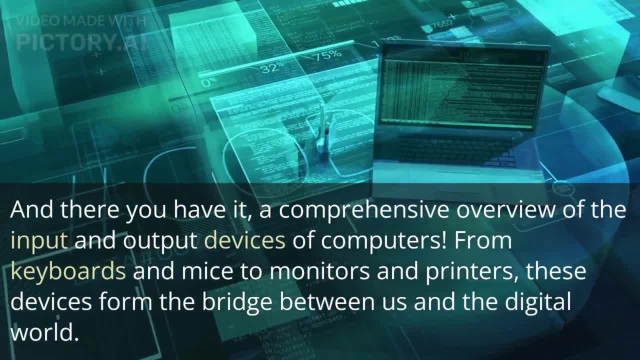 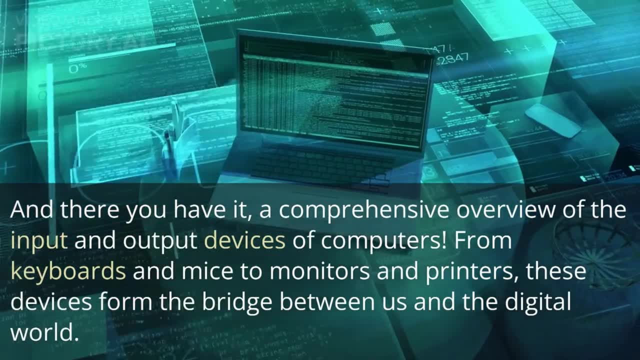 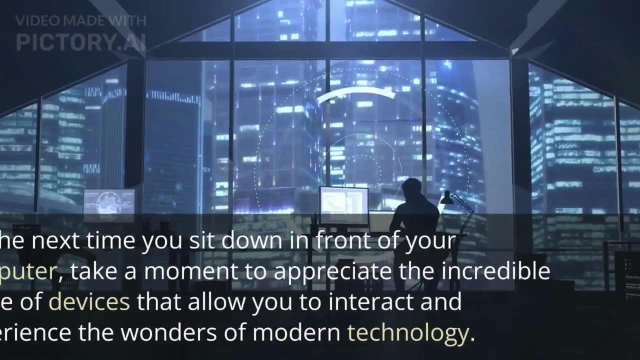 And there you have it: a comprehensive overview of the input and output devices of computers, From keyboards and mice to monitors and printers. these devices form the bridge between us and the digital world. So the next time you sit down in front of your computer, take a moment to appreciate the